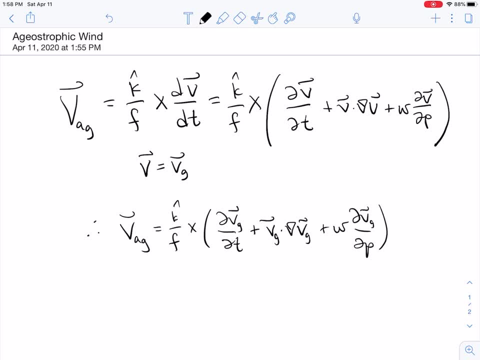 And we can do that by using the a-geostrophic wind vector, And we can do that by using the a-geostrophic wind vector, And we want to look at two of these elements in a little bit more detail to unlock some of the things that are contained within this a-geostrophic wind. 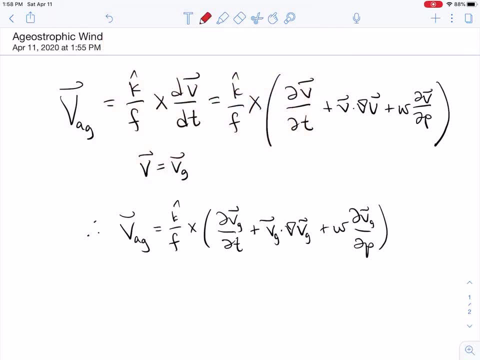 And so we are going to look at our first term here, which is our local wind tendency, And we'll allow us to determine the isallobaric wind. And then we are also going to look at our second term here, And our second term is going to allow us to look at the inertial advective wind. 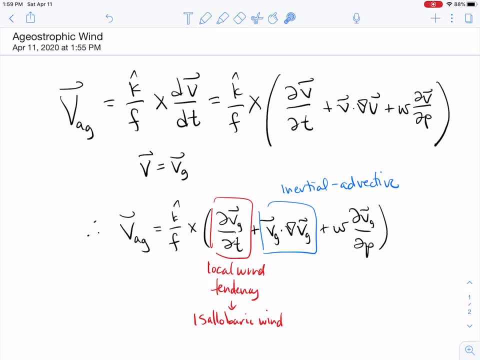 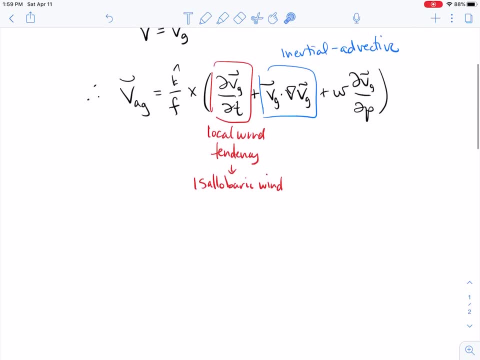 And then we're not going to do anything. but this third term is a convective term. that is part of our a-geostrophic wind, And so let's go ahead and do that, And let's go ahead and start with this concept of the isallobaric wind. 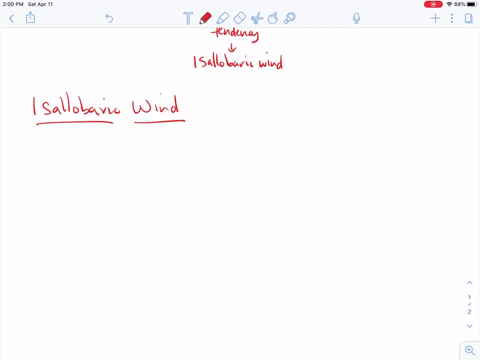 And so if you wanted to look up, we could look up what isallobaric means. And isallobaric means basically lines of equal pressure fall or rise, right, So of equal change in pressure, And so we can call out here just our isallobaric portion. 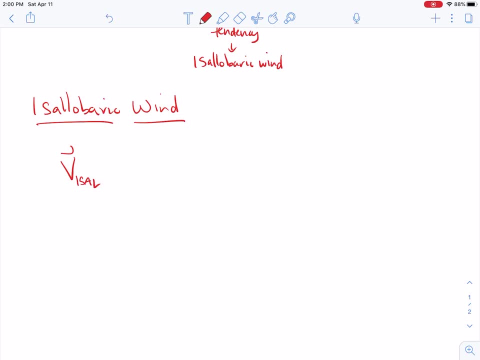 And so we can say that our isallobaric wind via isal equals k hat over f cross, dvg, dt. Now here, since we're using the geostrophic wind, we could substitute in for a geopotential height, such that we can change our equation or alter it to be k hat. 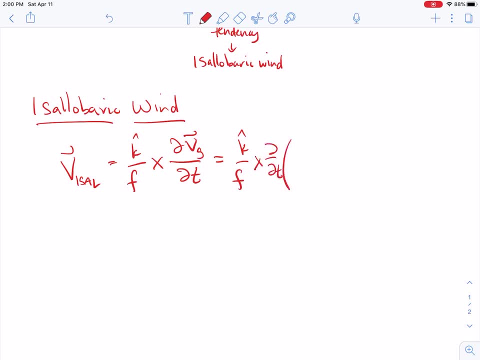 over f cross dvg dt, f cross dvg dt of the quantity k hat over f cross del phi, which will leave us with minus 1 over f squared del d phi dt. And so, ultimately, our isallobaric wind is going to relate to our vertical motion. 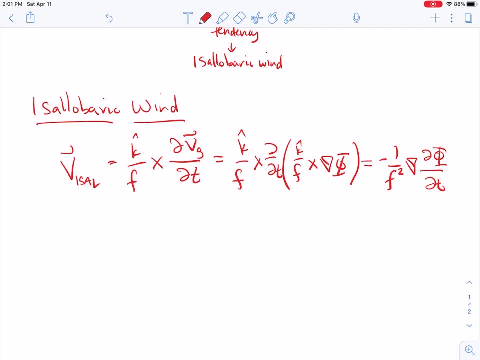 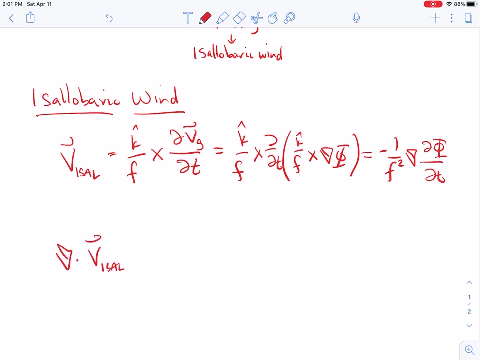 And so, if we go ahead and take the divergence of our isallobaric wind, we're going to take del dot v isal, such that we're going to get minus 1 over f? squared, del squared, d phi, dt. And again, what is d phi? 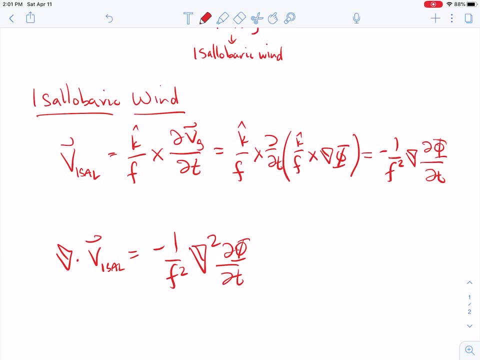 d? t Right, This is chi, This is our height change. We could also do the same thing for pressure falls, And so we could make a similar argument and say: it equals minus 1 over rho f squared, if we're going to do our conversion properly: del squared, dp dt. 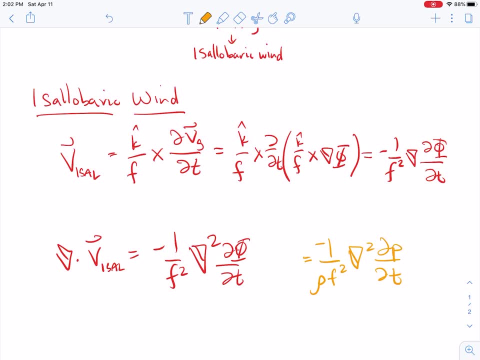 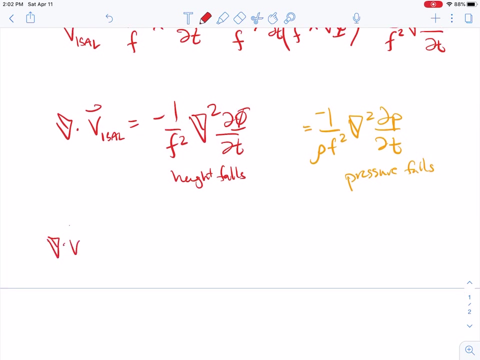 And so, whether we have pressure falls Or we have our more classic upper level height falls, the divergence of our isallobaric wind is going to help us determine where we're going to see convergence and then thus rising motion. And so if we have del dot v isall less than zero, that means then our term for our pressure. 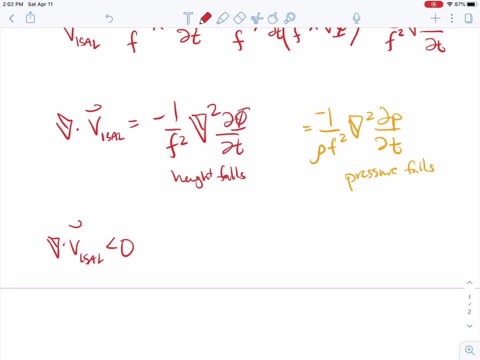 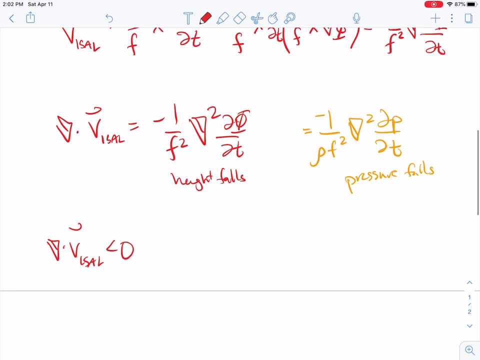 falls is going to have to be also less than zero. the whole term would be less than zero, such that we know we have the minus sign. so that would make it less than zero already, so that the combination of the rest must be less than zero. rho will be positive. 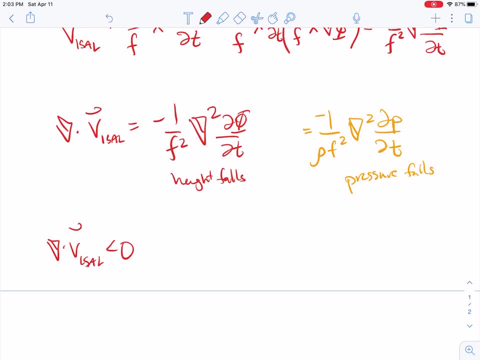 f squared will be positive del squared, the Laplacian will change the sign such that we know that then we should have dp dt also less than zero, And so that means pressure falls where we see convergence of the isallobaric wind. 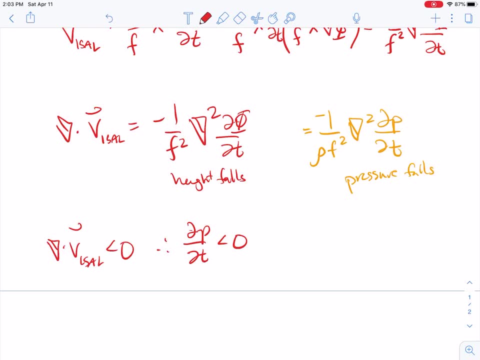 And so, subsequently, pressure falls are where we're going to see rising motion, And again, none of this should be surprising in the context of everything we've done this semester- but that this comes out of this a-geostrophic wind, and so it's important to remember. Similarly, 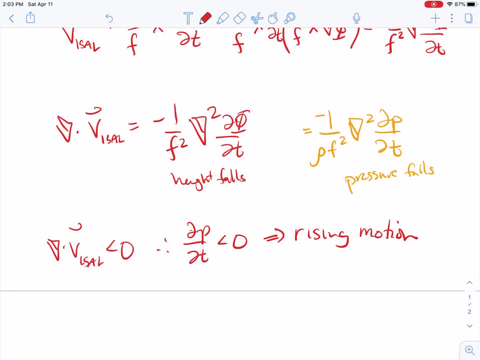 we could do the same argument for that divergence of the isallobaric wind being where we see pressure rises, we're going to see sinking motion And what we're really observing here is the development of where our new low pressure and high pressure are going to be. 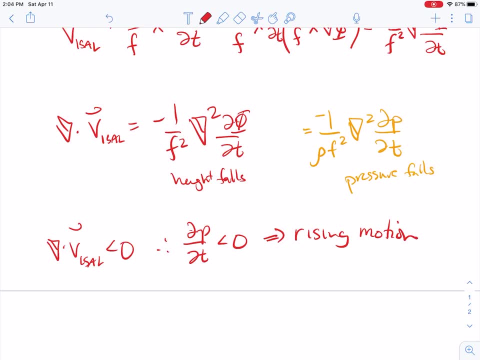 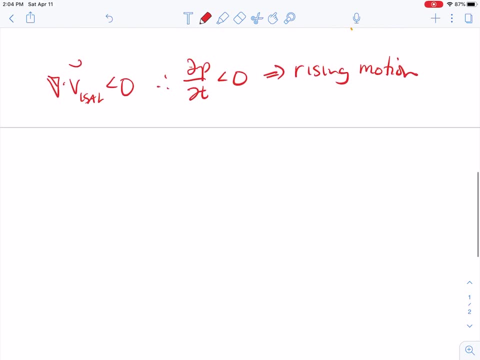 as we know, they constantly reconstitute themselves through time, Moving on to the inertial advective wind. this one is also a bit interesting and helps us to figure out a little bit about what's going on with our difluent areas of troughs. 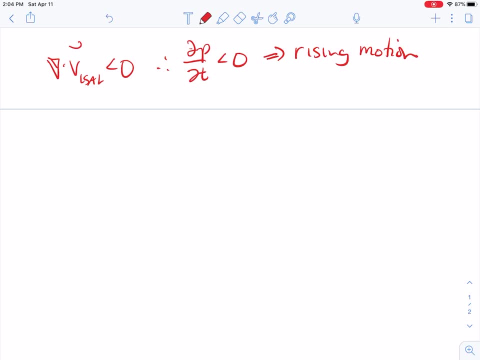 So let's go ahead and first write out some of our inertial advective equations, So the inertial advective wind, And so here we're going to call this VIA, and this equals our k hat over f cross. And now I am going to write out the terms here that we're. 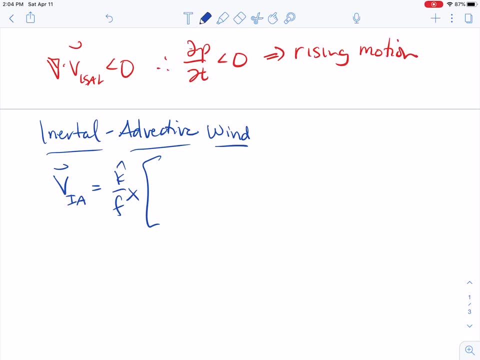 going to have in both our i and j components, And so remember that this is the advection of the wind by the wind, And so our i component is going to be ug du g dx plus vg du g dy i hat plus ug dv g dx. 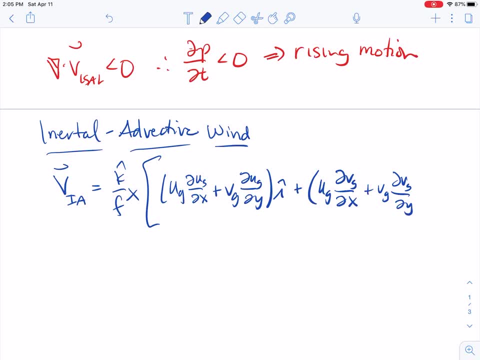 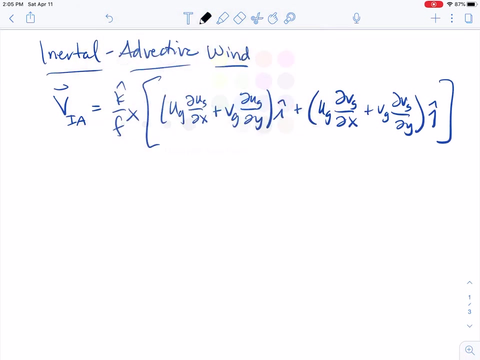 plus vg, dv, g, dy, j, hat, And there's our full inertial advective term. Okay, well, this is great, But let's go ahead and look at a drawing here related to our inertial advective wind. Let's go ahead and look at a difluent zone. 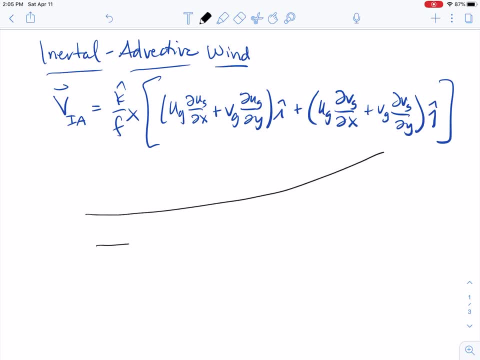 And so maybe this is 300 millibars and we have our normal difluent zone 912, 924, 936.. And so what we're really curious about here is what's going on in kind of this difluent zone here, And so we're going to look at it just right along this 924 contour here. 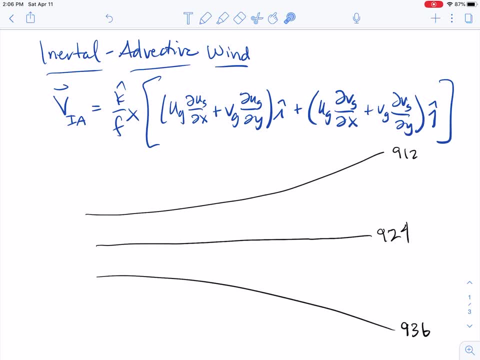 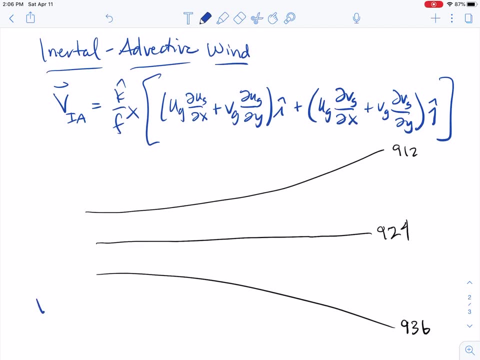 And so we can pare down our full equation here to look at just a subset. And so we're going to look at our inertial advective component. Here we've got an ordered frontic vいうこと unit and then we can look at the inertial according to our294- infinitive законч internacional. with the fn, we can draw the learners Anriver radius as 0.8 dash, we can closeこの, we can close this out here to theic And the calibrated. compare this parabola 3iling this잡ong here being v, i, a, as equal to k, hat cross or over f, x, sug, du, g, dx. And so we want to assess. we know that our ug here is going to be stronger here, weaker here. 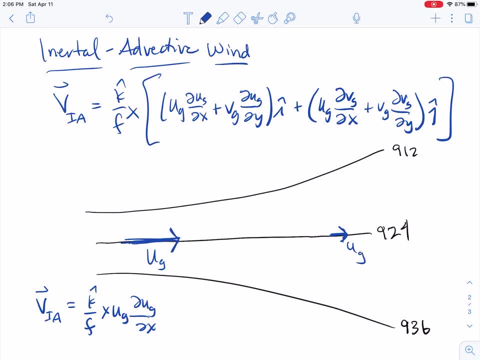 And so now we want to assess u, g, d, u, g, d, x, And so we can do that. So faster here, faster here, weaker here, as we go along in our positive x direction. So let me first indicate here our x and our y. 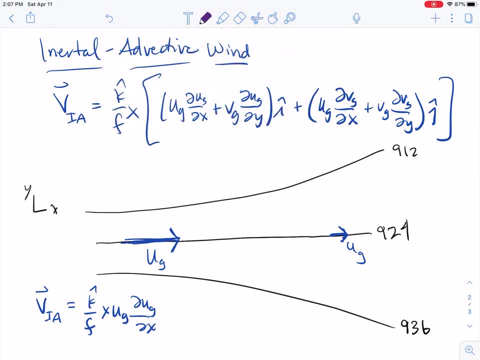 Okay, And so with our d, u, g, d, x term, right, what's happening? u g is decreasing as we go in increasing x direction Times. then u g is still positive, So that overall term is going to point back to the left. 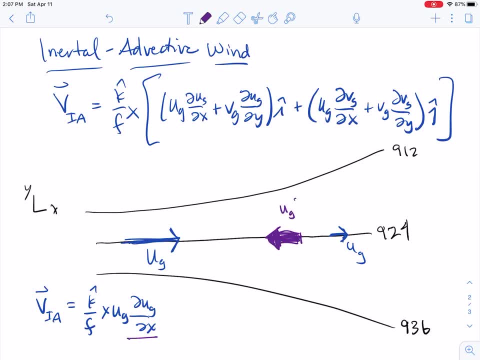 This is our u, g, d, u, g, d x term. Okay Again, because our wind speed is decreasing as we move in the positive x direction times a positive value. So d, u, g, d, x is less than zero, u g is positive, So that this whole vector is pointing to the west. 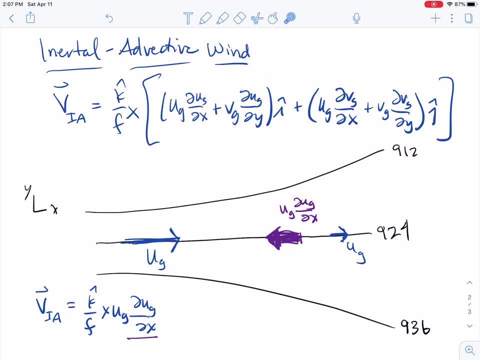 But now we need to use do our cross hat, k hat, cross v, right hand rules. This states that our inertial advective wind is going to point in which direction. That's correct. k hat goes up first. Curl your fingers to cross in the direction of u, g, d, u, g, d, x, And your thumb is going to point towards the south. 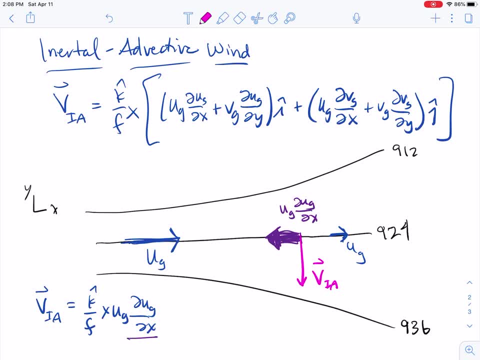 And this is going to be most pronounced right here along this 924 line, And so what that ends up meaning is that we are going to have a wind speed of 924.. So we are going to get convergent flow to the south and divergent flow to the north, according to our a geostrophic wind. 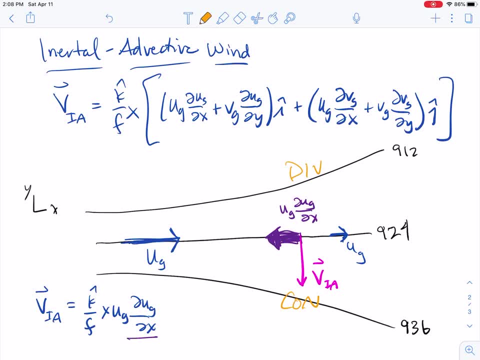 And so what this means for difluent areas is that the whole difluent area is not necessarily good for divergent flow. It is only this area to the north that is really good for divergence, And that's because divergence in natural coordinates Has two elements. 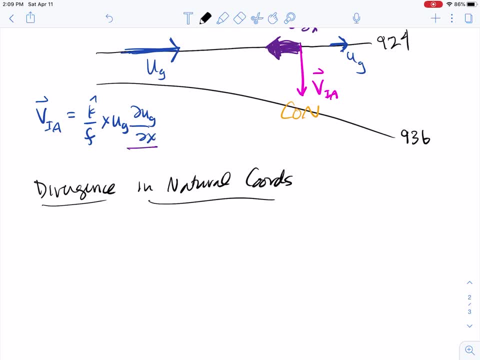 So just like we can do vorticity in natural coordinates, we can also do divergence in natural coordinates, And so we'll say: div here equals dv, ds plus v, d, alpha dn, And this first term here is speed divergence, And the second term here 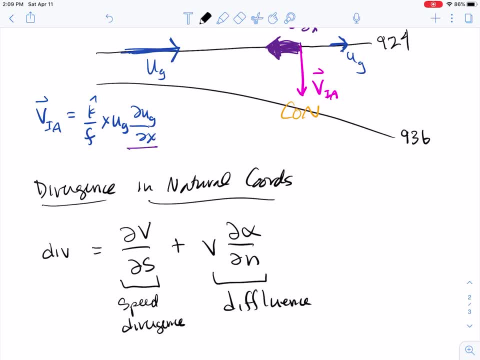 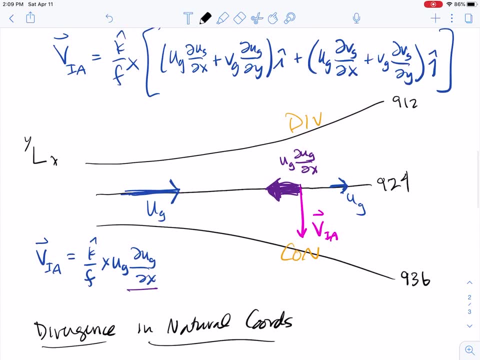 This is where we get that term: Difluence, or difluence Depending on how you talk about it: potato, Potato. So in general, we would consider this pattern that we drew up here to be difluent. Our heightlines disperse as we go. To the east. Difluence here will connect it And then a hexagon that we got disperse sporadically And the difference between two lines is pretty out. Sheng Brit, The difference between two lines is that it's recognised in white. 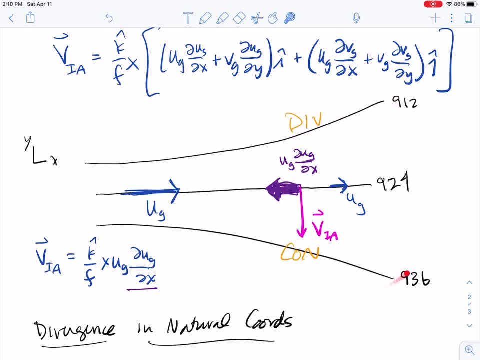 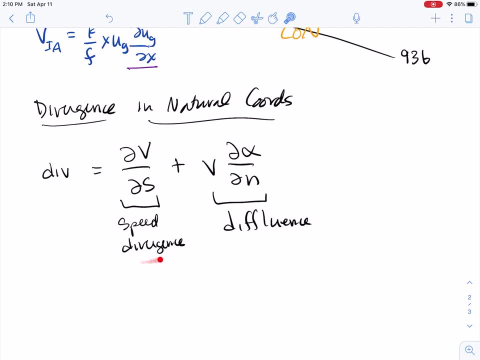 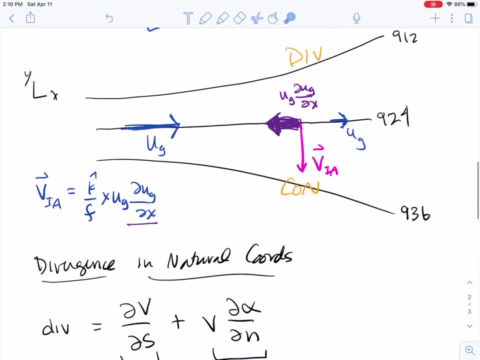 pattern here. Oftentimes, though, we talk about this difluent pattern as being good for divergence in and of itself, But, as we see in natural coordinates, we actually have this speed divergence term. that is a part of our overall divergence, And what is happening to the speed? 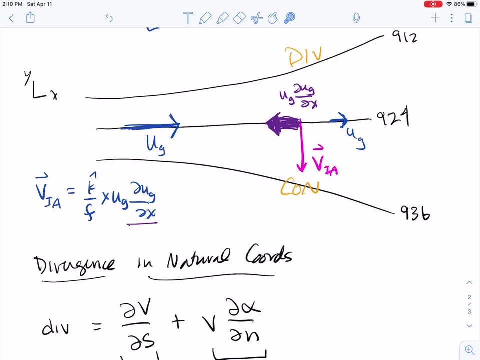 in this picture. That's right. it's decreasing as we leave and go into the difluent area, which that is going to cause convergence of flow in general. And so the question in this whole difluent pattern is what's going to win out? Is the speed divergence going to win out?